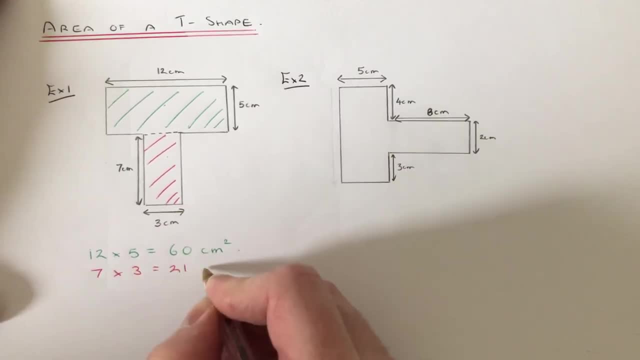 go 7 times 3, which is 21 centimetres squared. So once we've worked out the area of the two separate rectangles which make the T-shape, you just add these two numbers up now to give a final answer. So 60 times 21 is 81 centimetres. 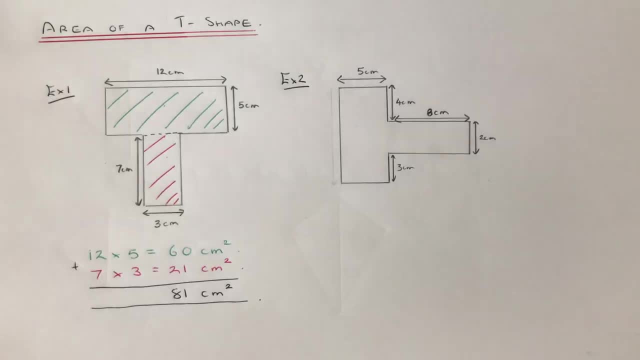 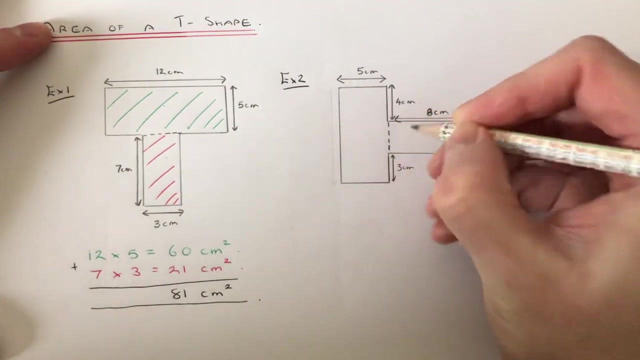 squared. So let's move onto example two then. So this one's a little bit trickier because we haven't got all the measurements that we need on our T-shape. So again, if we split the T-shape up into two rectangles like this: 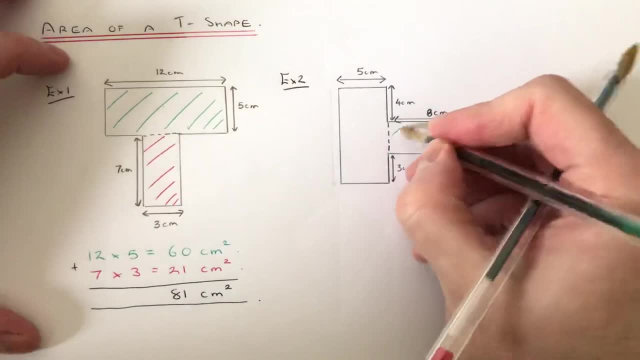 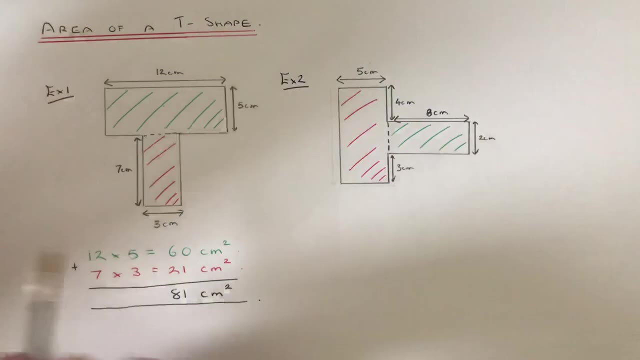 so let's colour this one in green and this one in red. so let's start with the green rectangle first, because we have the length and the width of the green rectangle. so again, we just need to multiply the 8 and the 2 together, so 8. 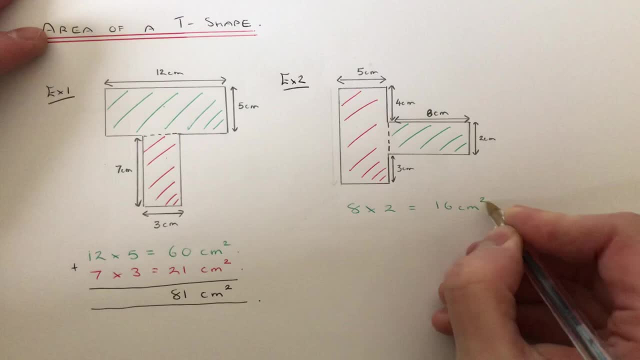 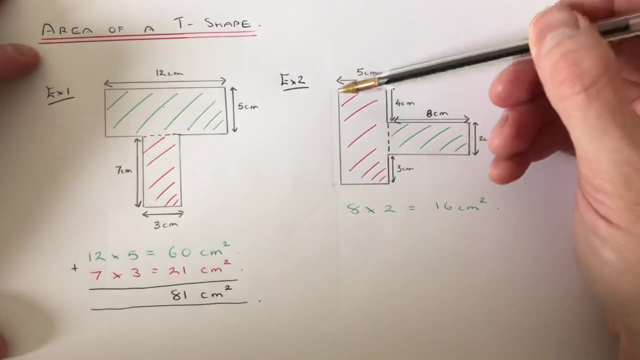 times 2 is 16 centimetres squared. so the red ones a little bit trickier to do because I haven't got the length of the red rectangle and you have the width okay, but we can find the length of that side there if we add up all the vertical. 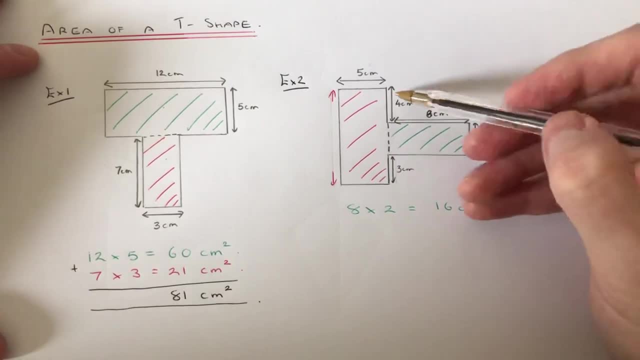 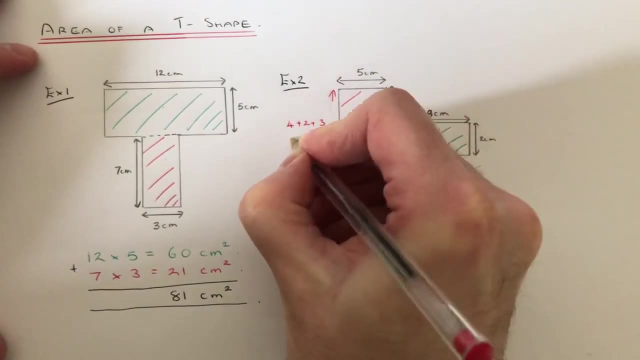 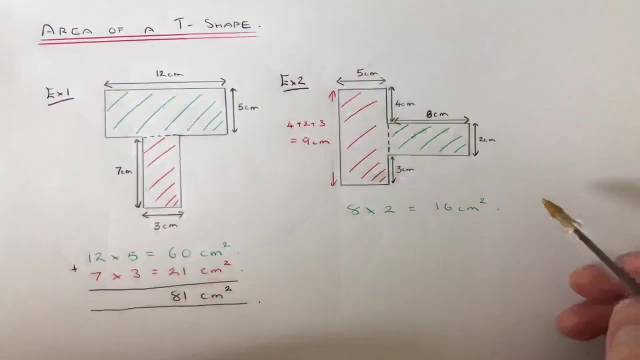 lengths up here. so we need to just add the four, the two and the three together, so that will give me nine centimeters. so the length of the red rectangle is nine. so again, if we just work out the area now by multiplying the nine by the five, so nine times five is forty five centimeters squared. so if we 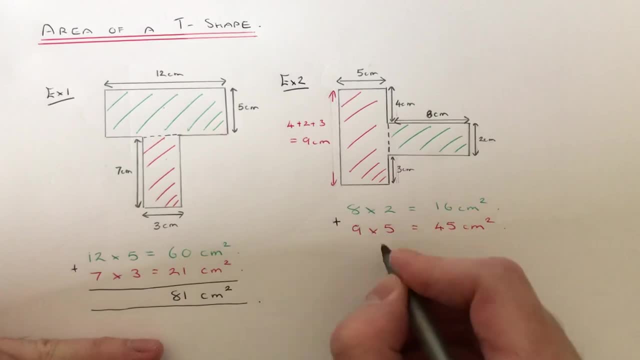 now worked out our two areas. so again we just need to add these two numbers up. so six add five is eleven. what four add one is five plus the one is six. so we get an answer of 61 centimeters squared. so if you like this video make. 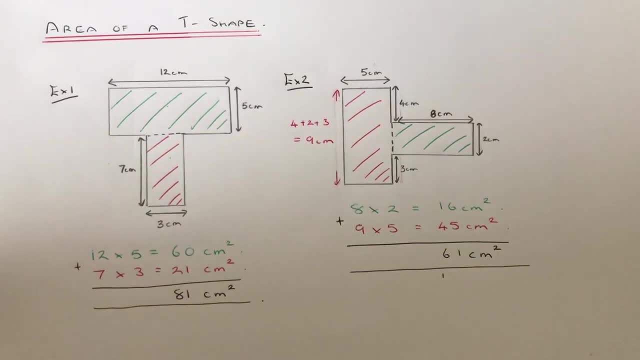 sure you like it and subscribe to my channel. thanks for watching, bye, bye.